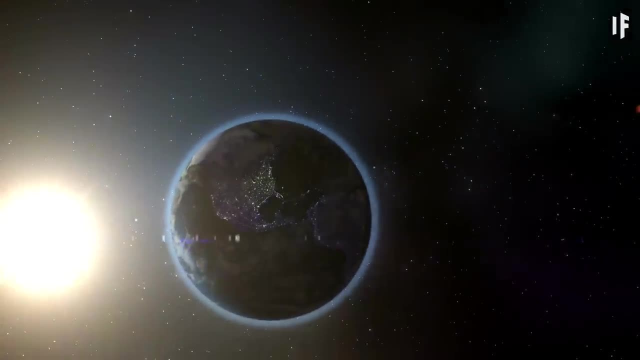 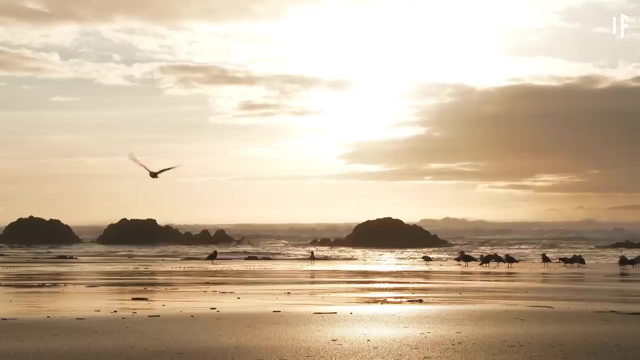 the greater the gravity. The greater the gravity, the stronger the pull. Gravity is the reason why Earth rotates around the Sun, why we experience high and low tide and why we can walk on this planet without floating away. Most importantly, though, 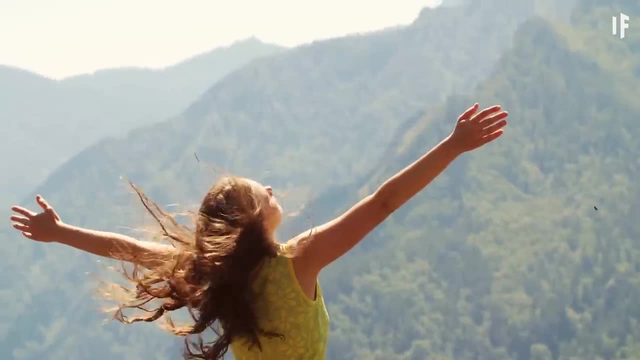 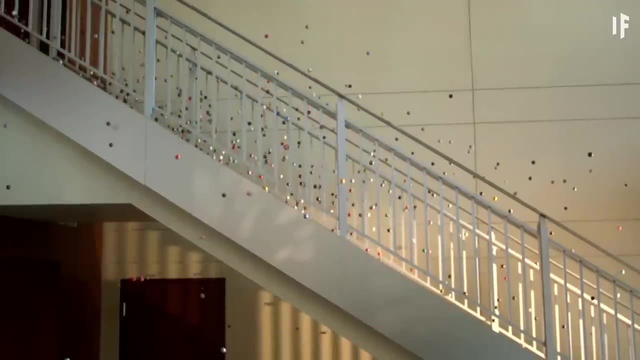 gravity secures our atmosphere, holding in the air we need to breathe. In fact, there are a lot of things we can thank gravity for. So many, though, that if we tried to list them all here, we'd probably end up with a video. 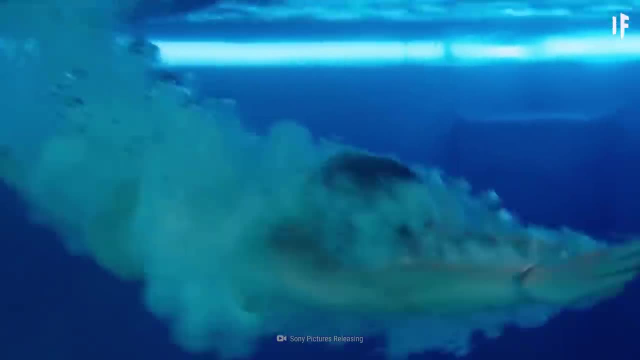 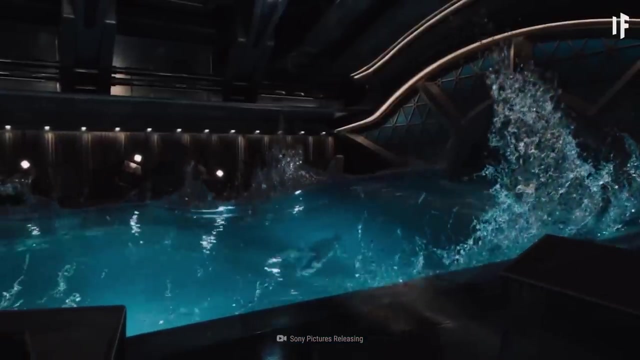 longer than Titanic. So just to give you an idea of how important gravity is, in a really, really short amount of time we're going to take it away from you, But not for too long, Just five seconds. Are you ready? 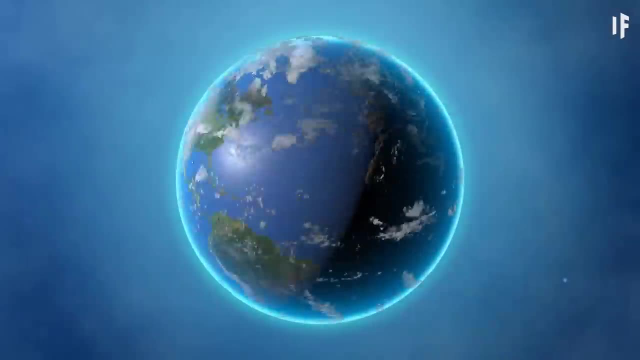 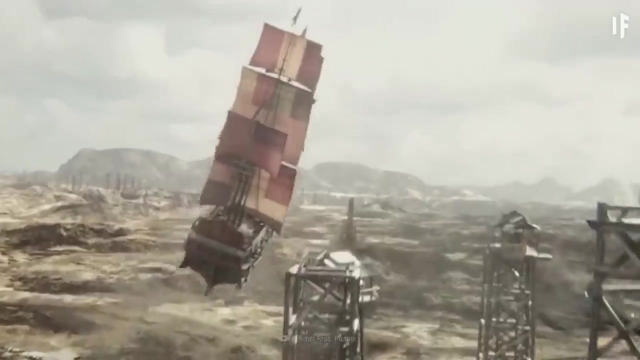 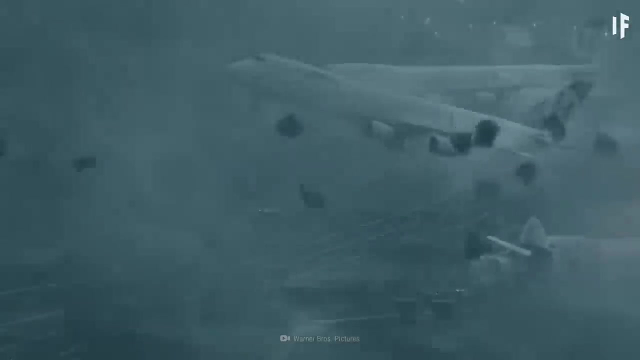 With the world still spinning at its usual 1,600 km per hour speed, everything that isn't secured firmly to the ground would go flying: Cars, boats, trains, planes. Well, obviously, but not like they normally do. More like this. 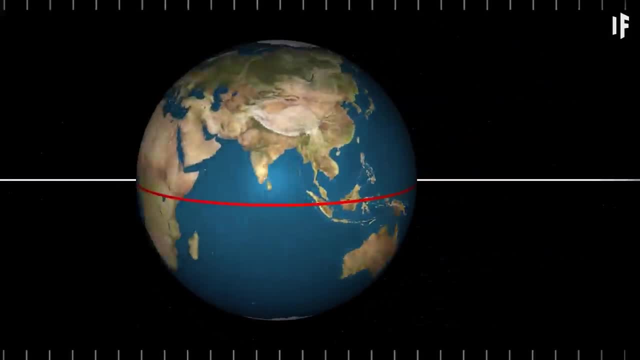 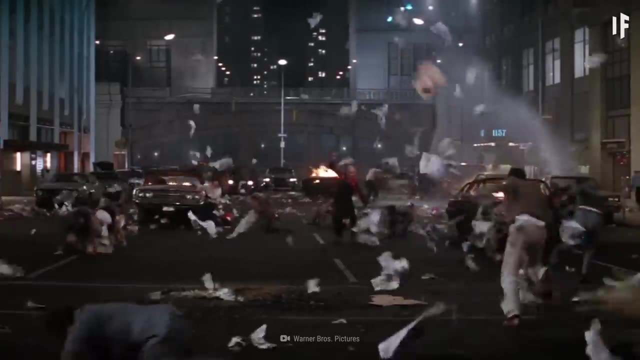 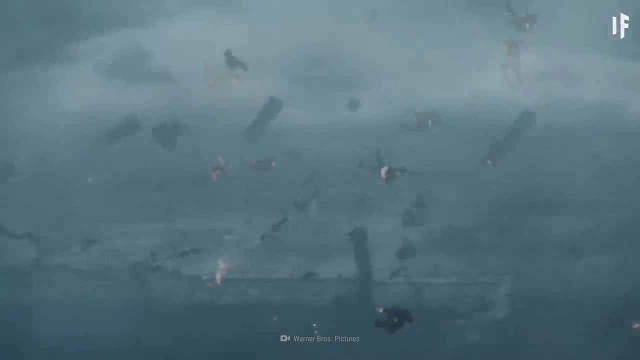 The Earth spins faster along the equator, so the impact of zero gravity would be felt hardest there. That means that in just five seconds you could be blown as far as 2.3 km in any direction. And not just you, There will be plenty of people. 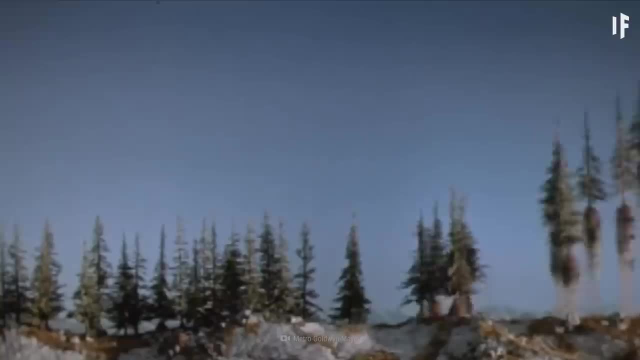 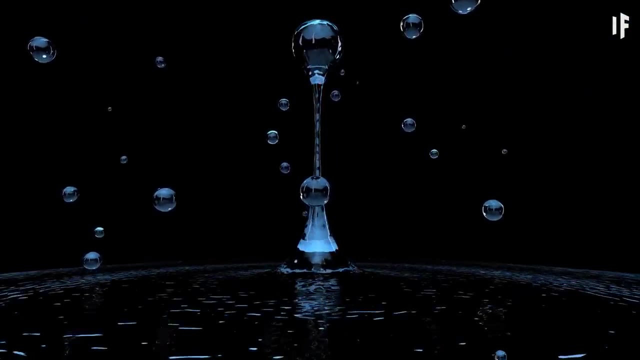 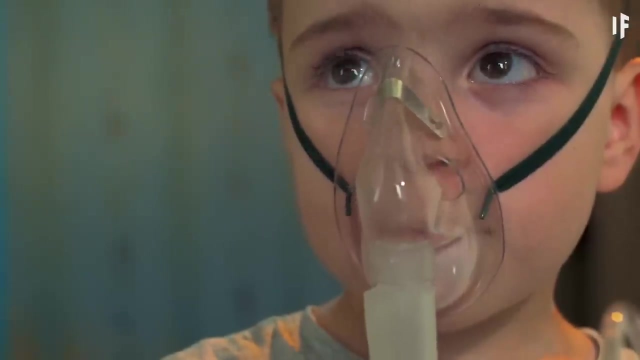 objects and animals to look out for, Not to mention trees, soil and mid-air floods from the world's ponds, lakes, rivers and oceans. At the same time, the gases in the atmosphere would drift out into space. Not only are we now losing, 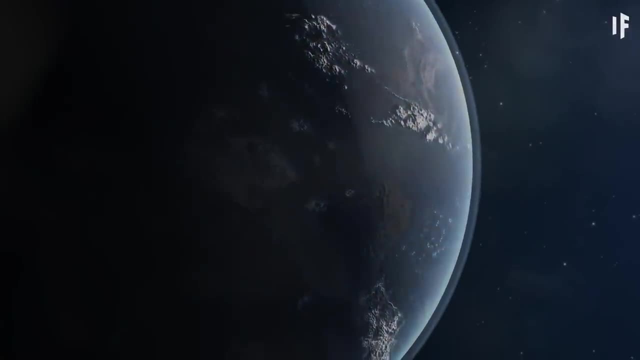 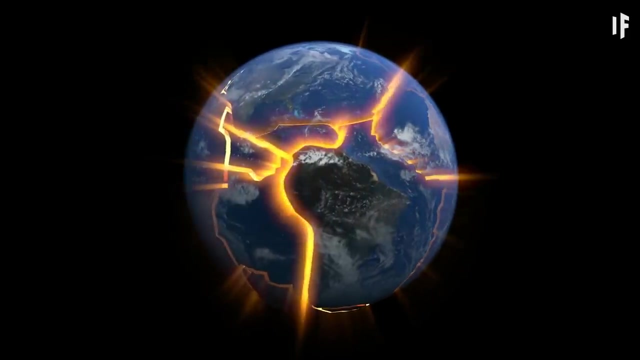 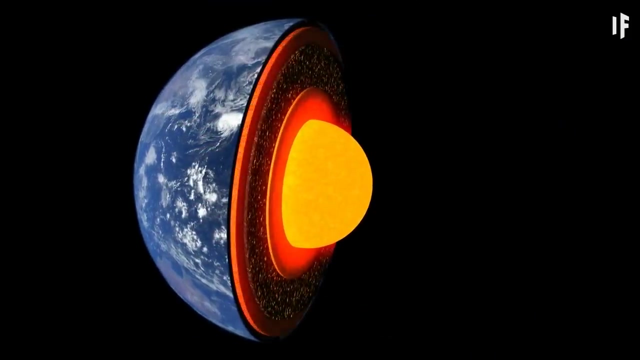 huge amounts of oxygen, but the sudden and sharp drop in air pressure would instantly shatter everyone's inner ears. And then there's the planet itself, which is literally held together by gravity. Without gravity, the pressure of the Earth's inner core would cause the planet to expand. 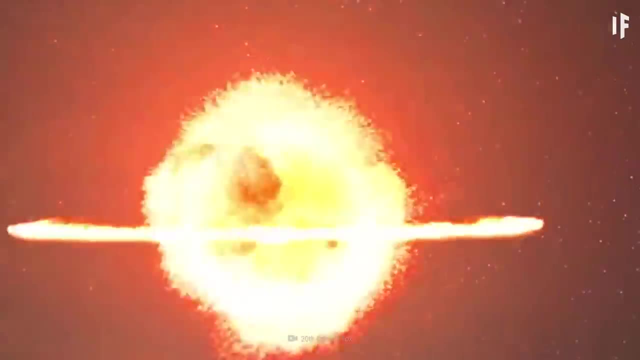 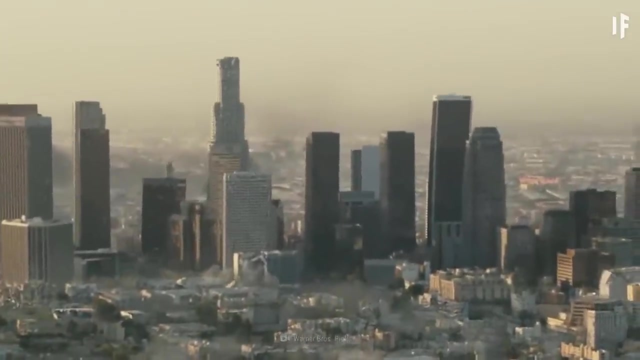 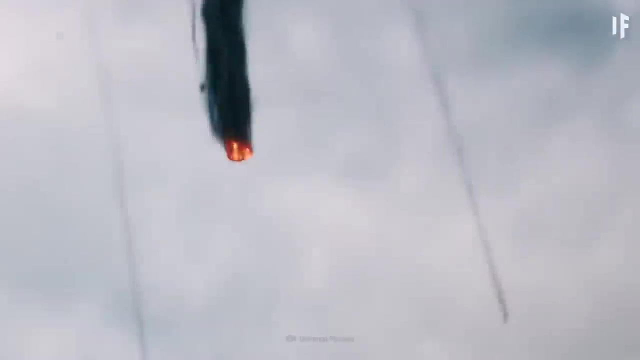 It's not like five seconds without gravity would cause the world to explode, but even a five-second expansion of the Earth's inner core would cause some major earthquakes and trigger huge volcanic eruptions. Add one more item to your list of dangerous things flying through the sky.